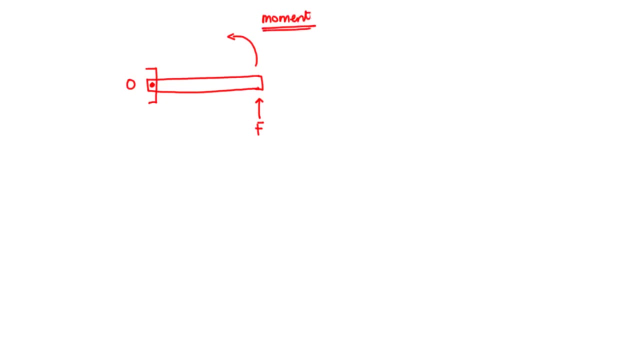 or simply moment, and basically that is what we are going to discuss today. now, the moment of the force f about the point o, which is represented as m, o is equal to the magnitude of the force, f times the perpendicular distance from o to the line of action of the force. 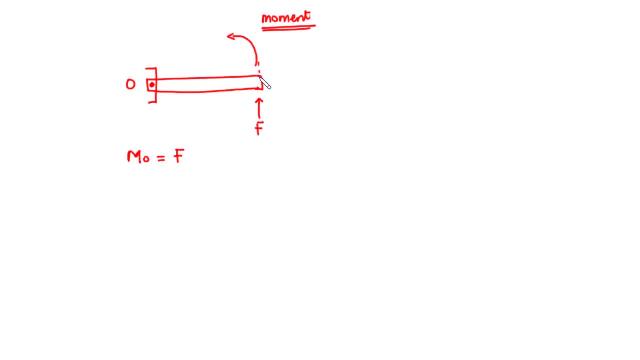 now we have the force applied here. so this is the line of action of the force and thus the perpendicular distance from o to the line of action of the force is this, and that is represented as d. so the moment of the force f about o is equal to the force times d. 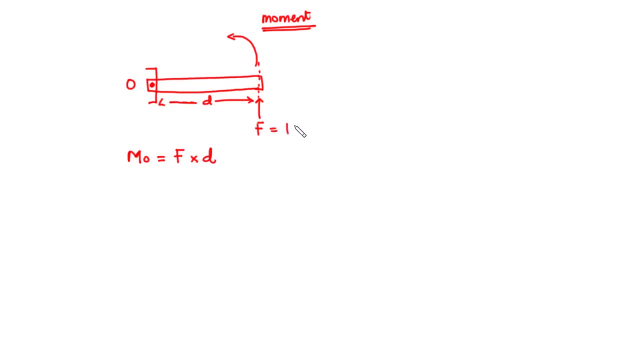 now, if f is giving us 10 newtons and then d is giving us 5 meters, then basically we are going to multiply these two values. now, because we are going to take the moment in the anti-clockwise direction, the force is going to be equal to the moment of the force f about o. 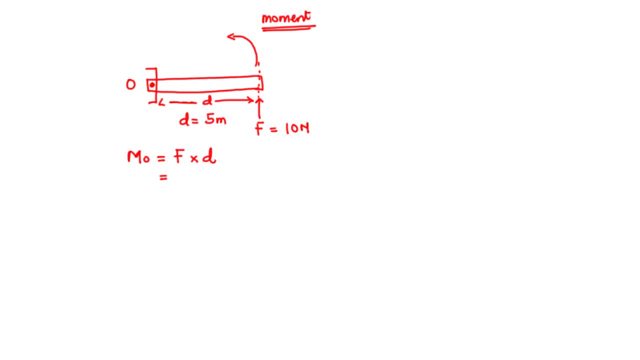 so we are going to have a negative magnitude now. on the other hand, if the moment is taken in the clockwise direction, then the force has a positive magnitude. so here we are going to have negative 10 because we are taking the moment in the anti-clockwise direction. 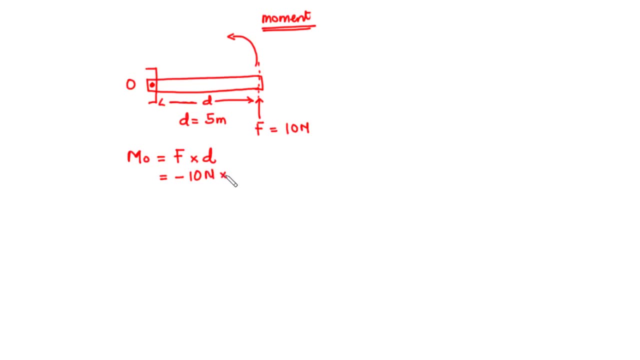 so negative 10 newtons times 5 meters, and that is equal to negative 50 newton meter. therefore, the moment of a force about a point is measured in newton meter, and in this example we took the anti-clockwise direction. now let's assume the case. 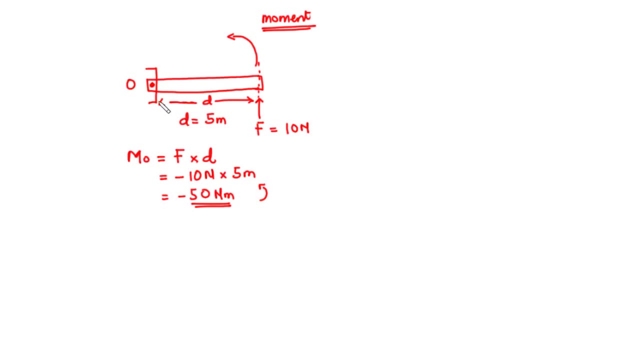 where we have the line of action of the force passing through o. so let's assume that we have this to be f2 and the line of action of this force is passing through o. now, since the line of action of this force is passing through the point in which you 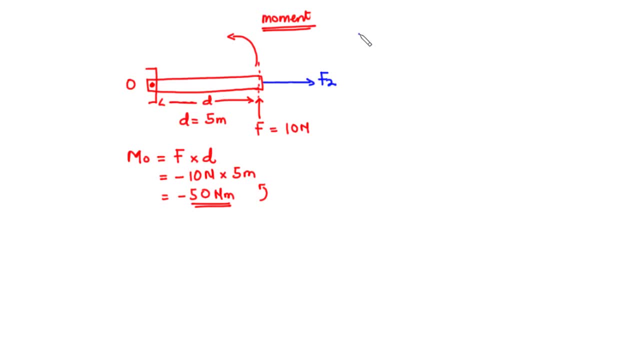 are going to take the moment about, then it means that for f2, the moment about the point o is equal to f2 times the perpendicular distance, which in this case is zero. now, because f2 is passing through o, it means that there is no perpendicular distance, so that is zero. therefore, the moment 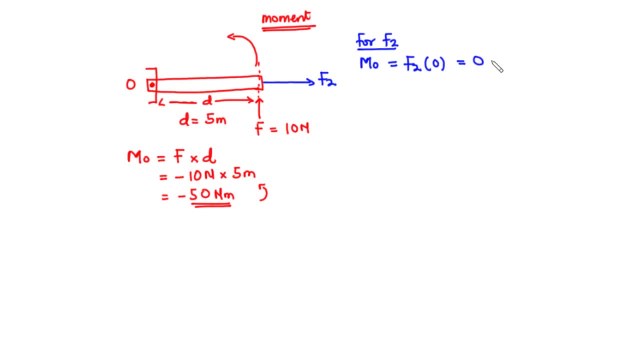 of f2 about point o is equal to zero newton meter. so actually there is no moment of f2 about o. again, let's consider a situation where the applied force or the line of action of the force is not directly perpendicular to the point you want to take the moment about, in this case about o. 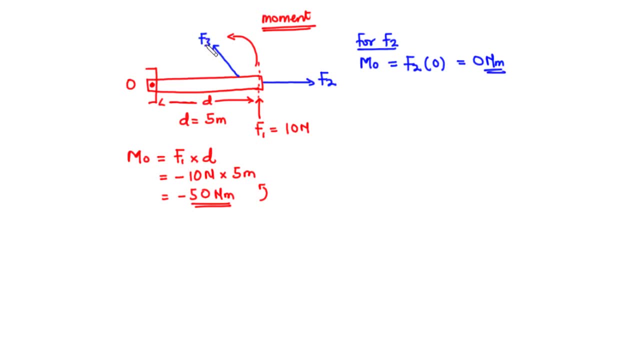 now, in such a situation, the best thing to do is to resolve the force into its x and y components. so we have this to be the x component of f3, so that is f3x, and then we have the y component of it, which is f3y. so after resolving this force into its 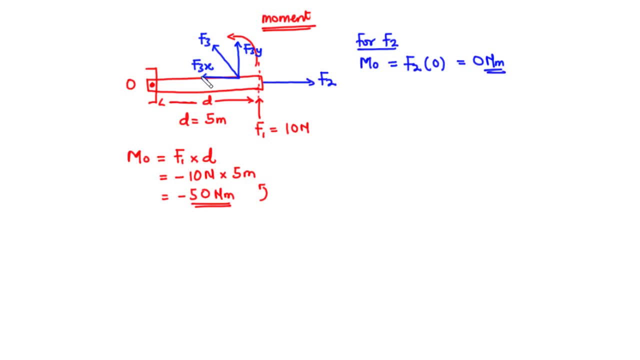 x and y components. we are going to take the moment of each of the individual force components about O Now. this is made possible due to the Varignan's theorem that allows you to resolve a force into its x and y components while you take the moment of the individual force component. 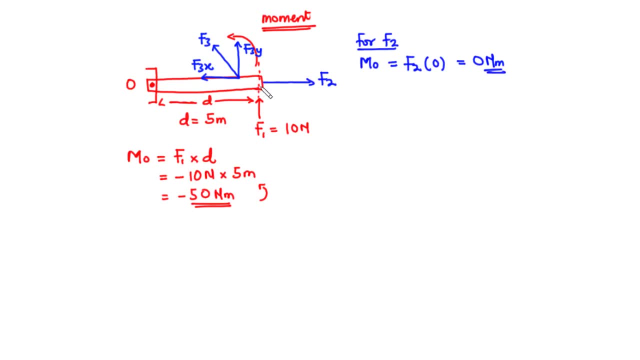 Now, at this point, we are going to neglect the width of the stick. We are going to assume that the width of the stick is very small, that we cannot account for that. Therefore, we assume that the line of action of F3x passes through the point O, which means that, since there is no 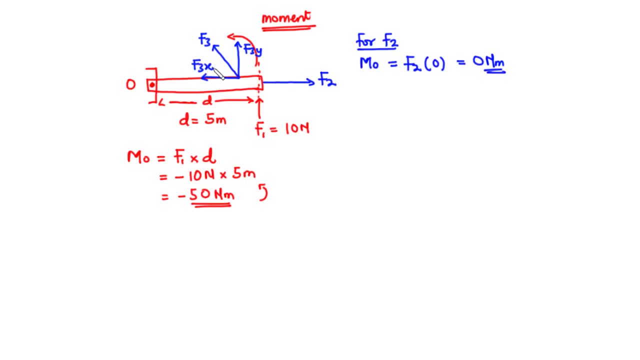 perpendicular distance, it means that the moment of F3x about O is 0.. Now, if there was a perpendicular distance- let's assume that there was a perpendicular distance- then what this primarily means is that we are going to take the moment in the anticlockwise direction. Therefore, this force 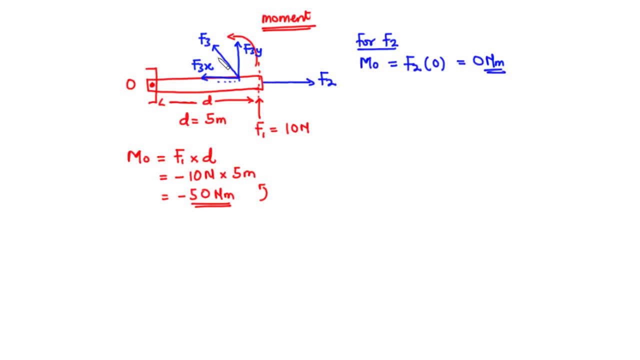 component is going to be negative. So in order not to confuse ourselves, let's say: for F3, we have moment about O to be negative, F3x and then times, because there is no perpendicular distance, so times 0. and then for F3y, we are also going to take the moment in the 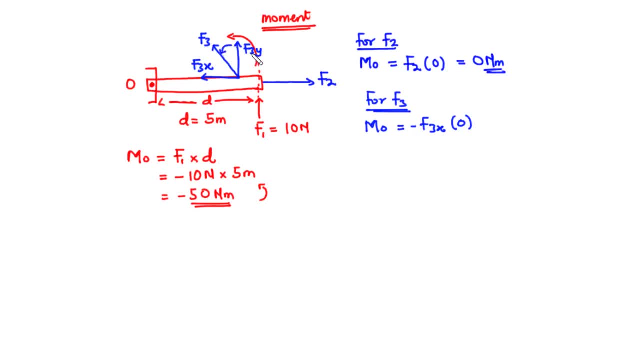 anticlockwise direction. So this is going to be negative, So negative F3y. and then times the perpendicular distance from O to the line of action of F3y. So that is from this point through to this point. So let's call that a. So let's say from this point through to this: 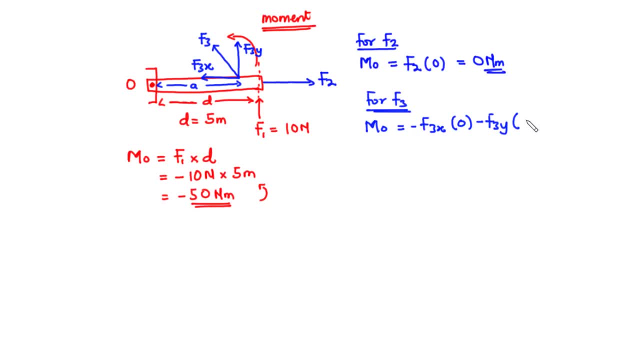 point is a, So times a. Therefore, the moment of F3 about O is equal to negative F3y a. So this is going to be negative F3y a. So this is going to be negative F3y a Newton meter. so always you need to understand that the force or the line of action of the force 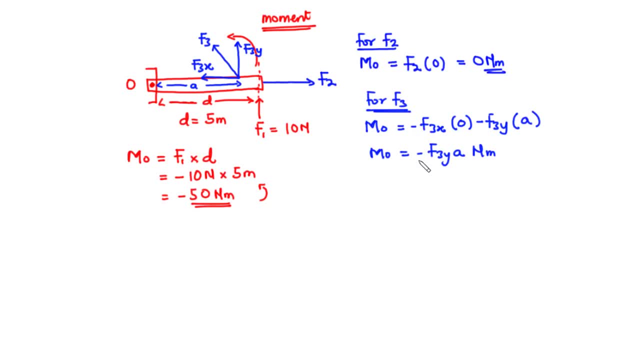 should be perpendicular to the point you want to take the moment about and basically, that is what moment of a force is all about. now, having got this, let's try a few examples. so let's take the first example: determine the moment of the force about point o. so this is point o and we are going. 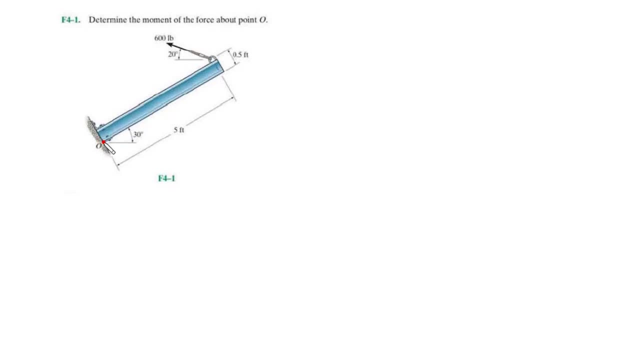 to determine the moment of this force? about this point: now, when you look at this question, you realize that this force is not directly perpendicular to the point o, or, better still, to the axis containing o. so in that case, the best thing to do is to resolve this force into its x and y components. 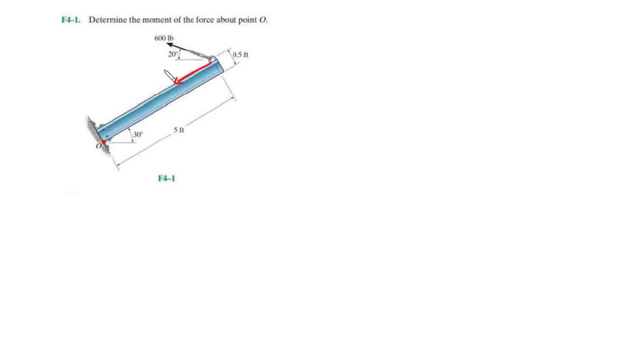 so we have this to be the x component of the force, and then this to be the y-component of the force. notice that we have this force to be 600 pounds. now let's change the unit toows, and then we have the length to be in meters. so we have 600 newtons, 0.5 meters, and then the length to be in meters, and then we have 600 newtons, 0.5 meters. so we have 600 newtons, 0.5 meters, one nuts. and then we have the curve to be in v界 records. So we have 600 hussle minuten. usar los geil omítosE Ü xz-jatüs. byating the sum of measures present in this model nats the length, target distance. we stack premiums in the good is by taking gust. пост regiment opneum spcom. 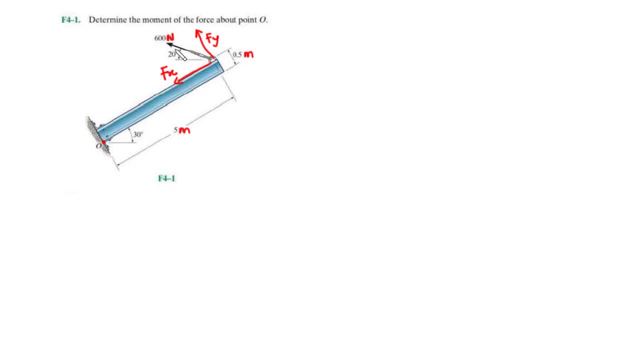 than 5 meters. So after resolving the force into its x and y components, you realize that the angle between this line and the positive x axis is 30 degrees, And then these two angles are alternating angles. So what this primarily means is that if this angle is 30, then this: 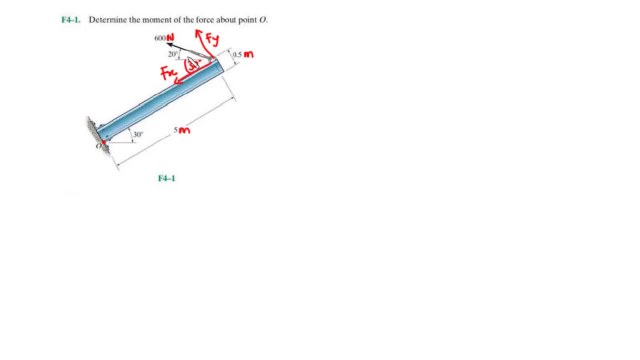 angle is also 30 degrees. So the full angle between these two forces, that is, the 600 alternating force and then its x components, is 50 degrees. So the angle between these two false components or these two forces is 50 degrees. Therefore, if you want to find 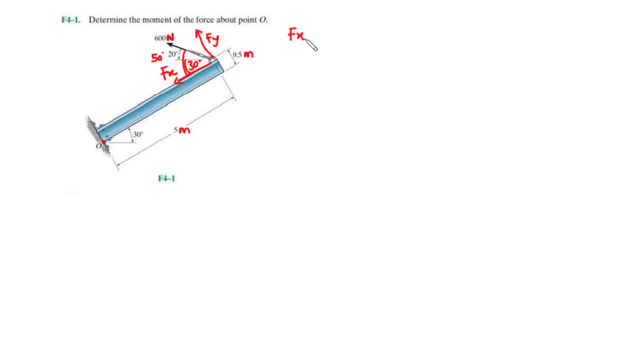 f x and then f y. we have: f x equals 600 times cosine of 50. So 600 cos 50.. And then for f y, That's basically going to be 600 sine 50. Now, 600 cos 50 gives 385.67 Newtons. 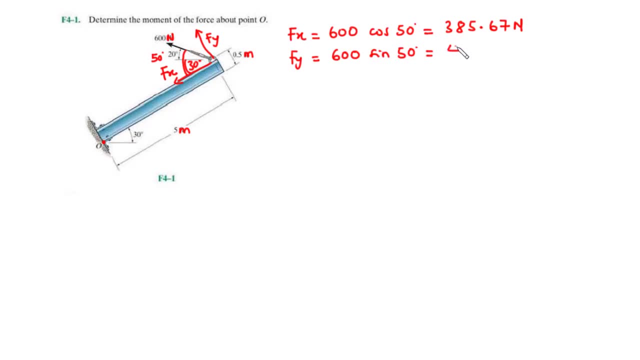 And then 600 sine 50 also gives 459.63 Newtons. So at this point we are going to take the moment of each of the force components, Which are Fx and then Fy about O. So, starting from Fx, we are going to take the moment in the anticlockwise direction. 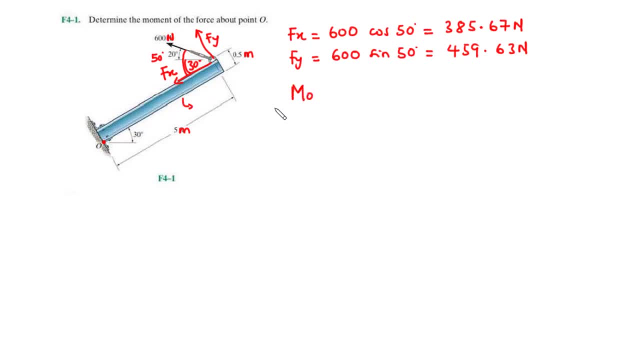 Which means that the moment about O is equal to. Since we are going to take Fx in the anticlockwise direction, It becomes negative. Fx Times: the perpendicular force, The perpendicular distance from O or the axis containing O. Now we have this to be O And the perpendicular distance from O or the axis containing O. 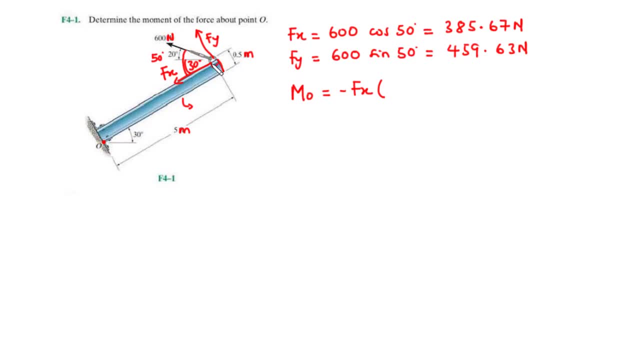 Is 0.5 meters. So this is the perpendicular distance from O to the line of action of Fx. So that is 0.5 meters. So we have times 0.5 meters. And then for Fy, We are also going to take the moment in the anticlockwise direction. 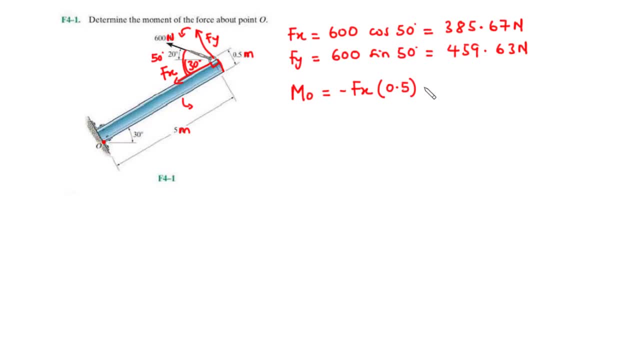 So that's also going to be negative, So the force becomes negative. Fy Times the perpendicular distance from O or the axis containing O. So this is the perpendicular distance And that is 5 meters. So times 5. Now let's substitute the values of Fx and then Fy. 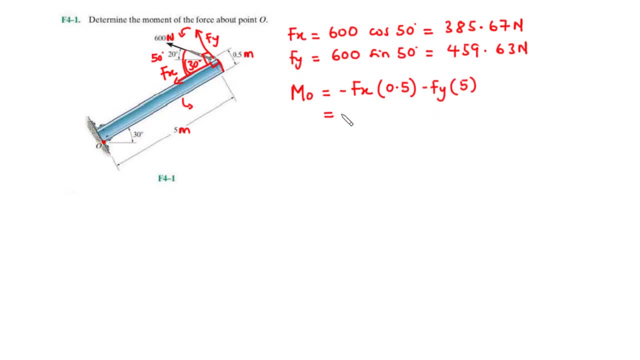 Into this equation. So we have negative Fx, And then Fx is 385.67 Newtons Times 0.5, And then minus Fy, Which is 459.63, Also times 5. Now let's simplify this. So negative 385.67 Newtons times 0.5. 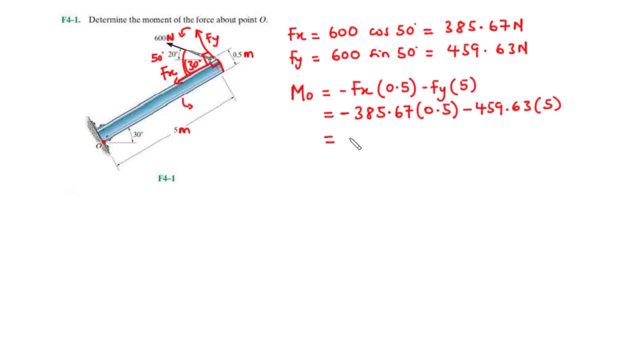 Gives negative 192.835, And then negative 459.63 times 5 Also gives negative 2298.15. So when you subtract this value from this, you have Negative 2490.985 Newton meters. Now we can simplify this as negative 2.49 kilonewton meters. 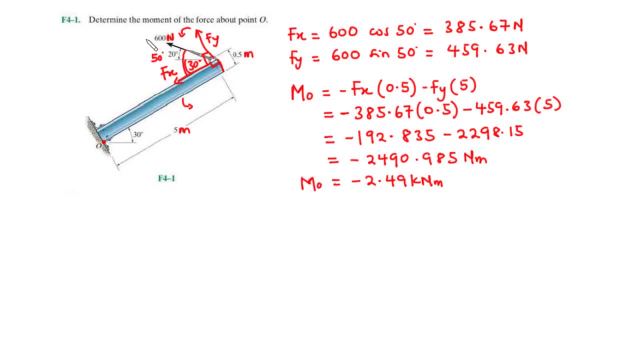 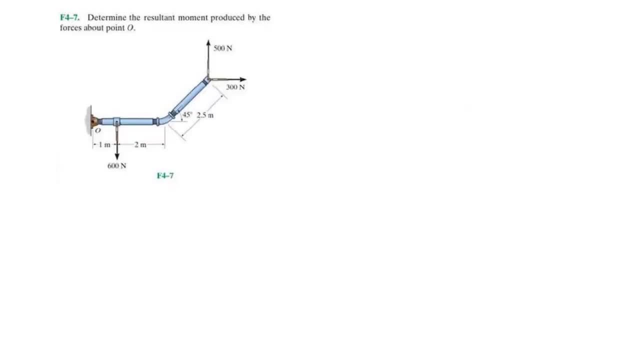 So that is the moment of the force about point O. Now let's take the second example. Now to this example, We are going to determine the resultant moment produced by the forces about point O. Now, looking at this question, you realize that we have more than one force. 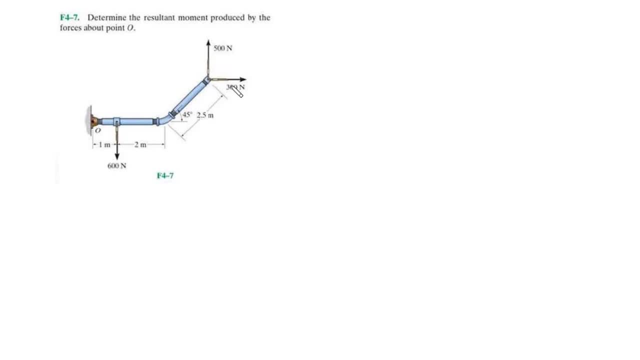 We have 600 Newtons, 500 Newtons And 300 Newtons. Now we are going to determine the resultant moment produced by forces, Or the forces about point O. So this is point O. So we know that to find the moment of a force about a point, basically we are going to multiply. 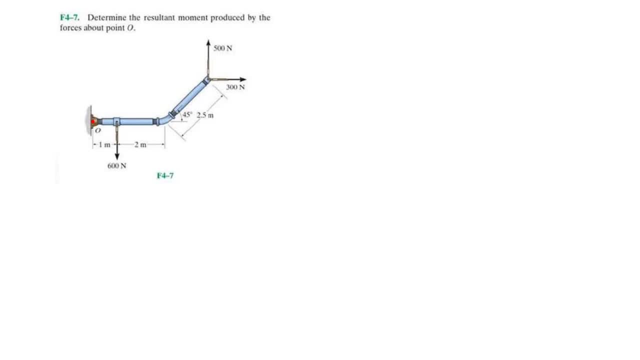 The magnitude of the force by the point O, by the perpendicular distance from the point you want to take the moment about, to the line of action of the force. So basically, we are going to find the moment of all these three forces about O. So let's start off with the 600 newtons force. So we have the magnitude to be 600 newtons. 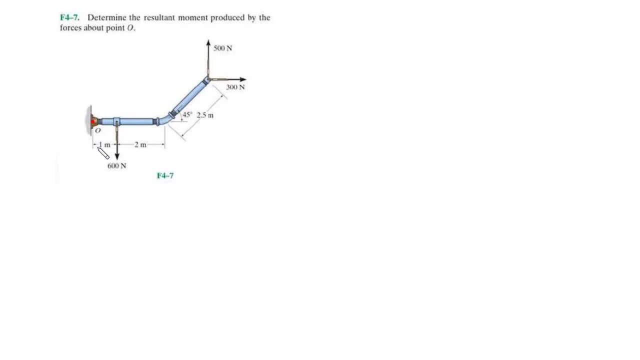 and then we have the perpendicular distance to be one meter from O to the line of action of this force. So this is the perpendicular distance, one meter, and then we are going to move in the clockwise direction, in the clockwise direction. So basically it is the force times the perpendicular. 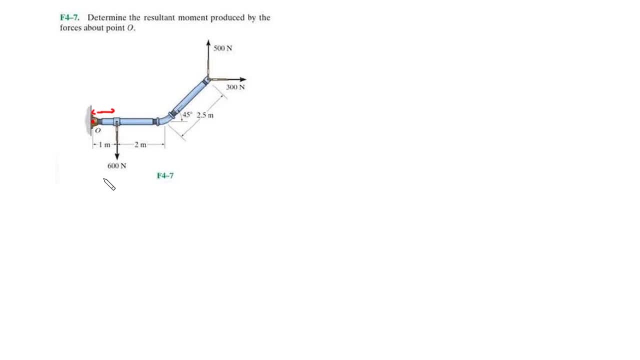 distance. So the perpendicular distance is one meter. that is considering this force. and then, because we are going to take the clockwise direction, this force is going to be positive. Now let's move on to the 500 newtons force. You realize that the line of action of this force can be extended through to this point. 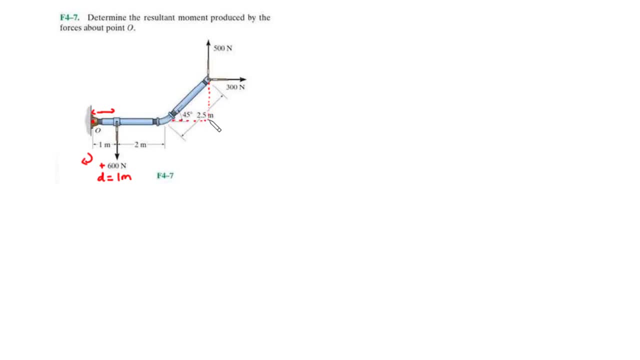 and if you want to find the perpendicular distance from O to the line of action of this force, you realize that that is going to be one plus two, plus the horizontal distance from this point through to this point. So how do we find the horizontal distance from? 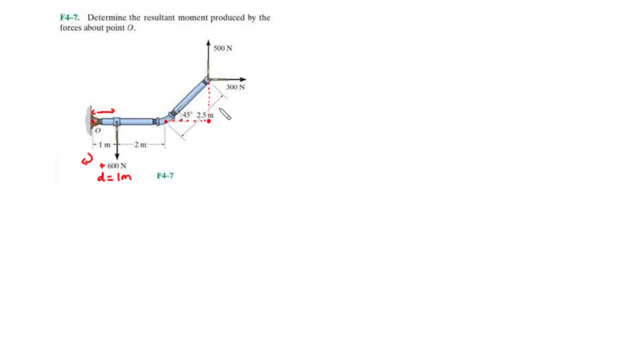 this point through to this point. Now you realize that we have this length or this distance to be 2.5 meters. So if you want to find the horizontal distance between these two points, then it's going to be 2.5 times cosine of this angle. So, considering this force, which is 500,. 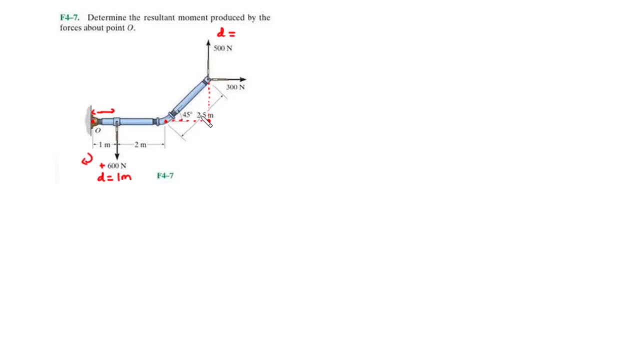 the perpendicular distance from O to the line of action of this force is going to be 1 plus 2 plus 2.5 times cosine of this angle, And then notice that we are going to take the moment in the anti-clockwise direction, So that's going to be negative. 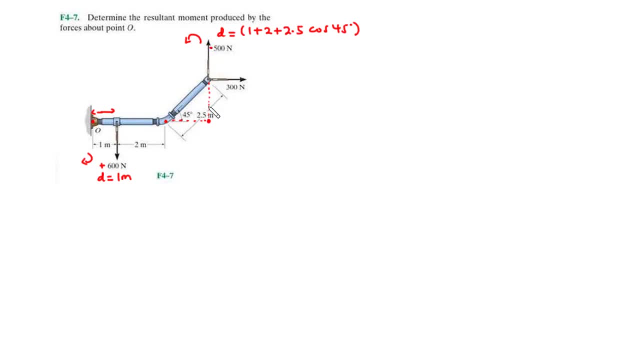 So that's going to be negative. And then notice that we are going to take the moment in the anticlockwise direction, So that's going to be negative. So this is the line of action of the force, and then this is the perpendicular distance from O. 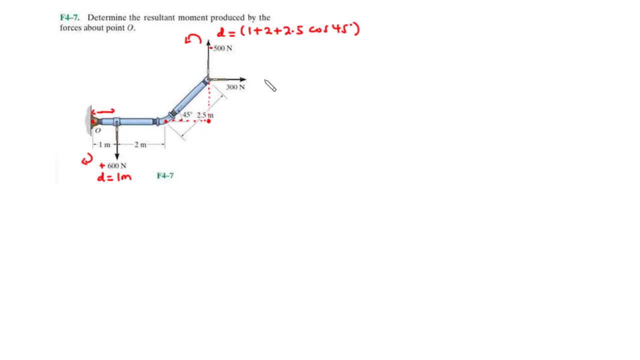 So we are going to take the anticlockwise direction. Now to the 300 Newton force. the perpendicular distance from O to the line of action of the force is this vertical distance or this vertical length. So if you want to find this vertical distance, 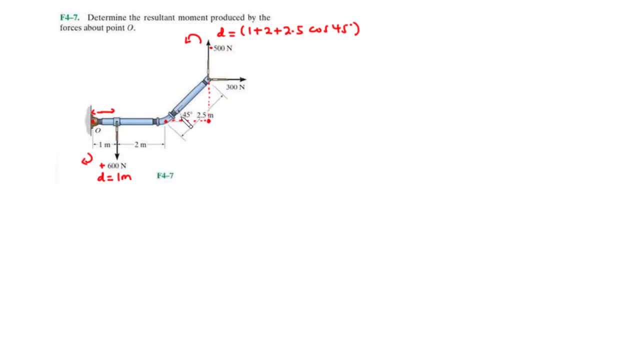 then it's simply 2.5 times cosine of this angle. then it's simply 2.5 times cosine of this angle. So, considering the 300 Newton force, we have d to be 2.5 times sine 45. And that is the perpendicular distance from O to the line of action of this force. 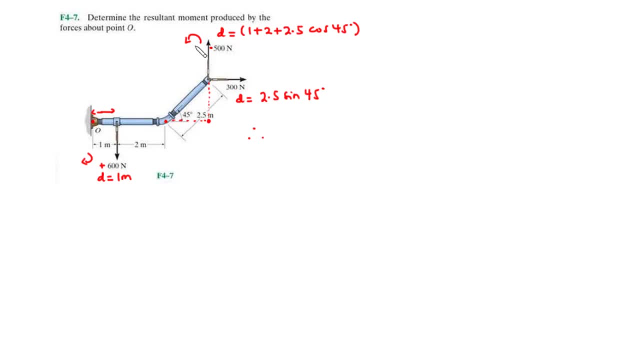 Therefore, the resultant moment produced by the forces about O is equal to the force of the angle. Therefore, the resultant moment produced by the forces about O is equal to the force of the angle. Now, even before that notice that we are going to take, 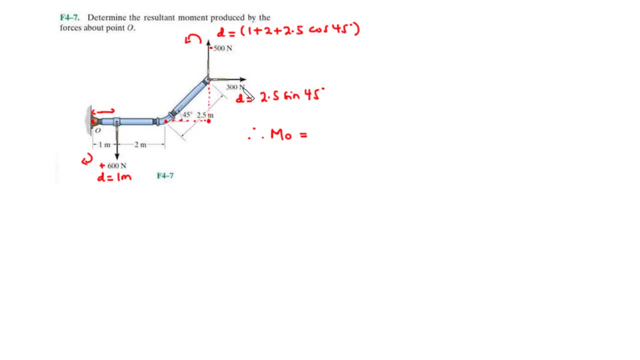 the moment of this force about O in the clockwise direction. So it's going to remain positive. We are going to move in the clockwise direction. So the moment or the resultant moment produced by the forces about O is simply 600 times 1 and then minus. 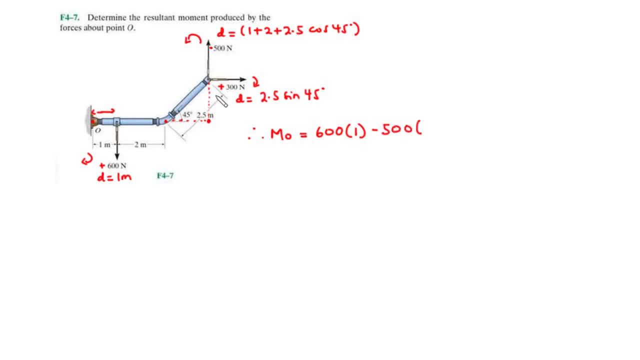 500 times. Okay, so that that's going to be 900. So that's only going to really cause us 잊화 е ش bell 500 times Now, 2.5 cos 45 is 1.7678.. So 1.7678 plus 3 is going to be 4.7678. Plus 3 is equal to 400 timesрат H國. 500 plus 400 times left in du Syndrome. 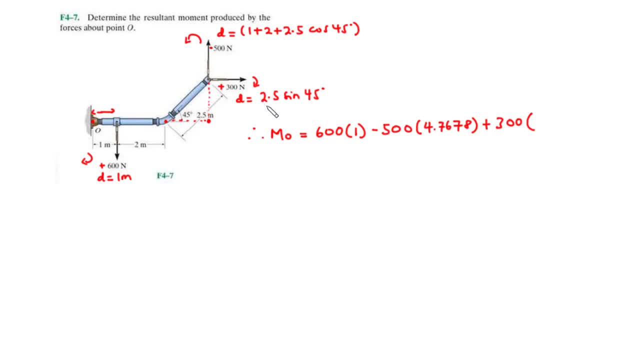 times 2.5 sin 45.. Now 2.5 sin 45 is also 1.7678.. Now let's simplify this: 600 times 1 is still 100.. Negative 500 times 4.7678 also gives negative 2383.9.. And then plus 300 times 1.7678. 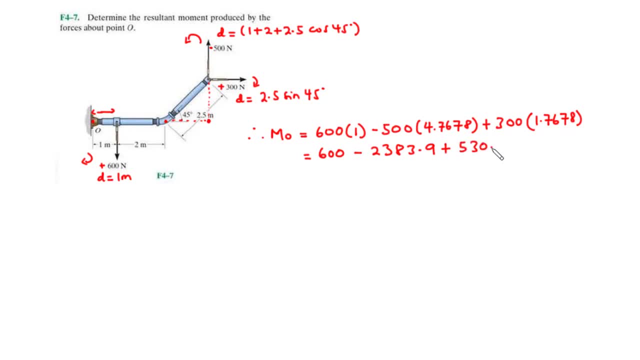 gives 530.34.. So simplifying this, we are going to have negative 500 times 4.7678 is also negative 2383.9.. And then plus 300 times 1.7678 is negative 1253.56 Nm. And then we can simplify this as negative 1.25 kNm. So that is the resultant. 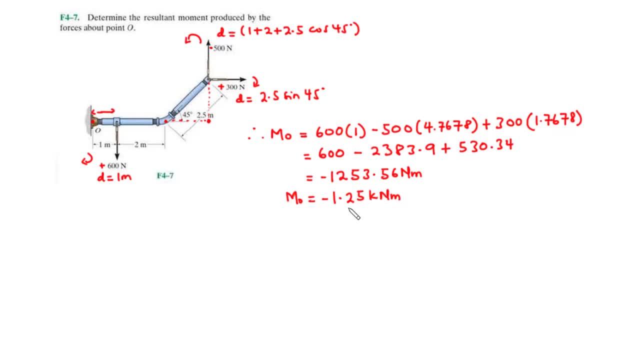 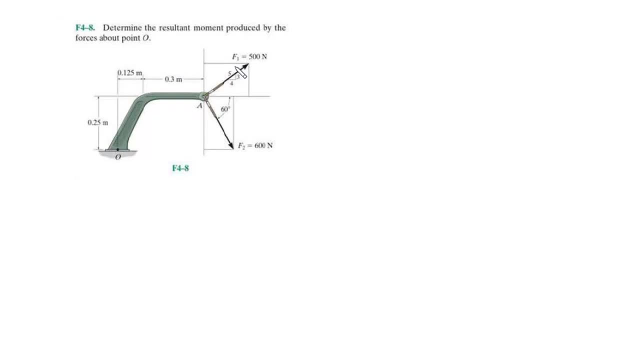 moment produced by the forces about point O. Now let's try the last example. So to the last example. we have two forces, F1 and F2. And then we are going to determine the resultant moment produced by the forces about point O. Now for F1, instead of an angle. 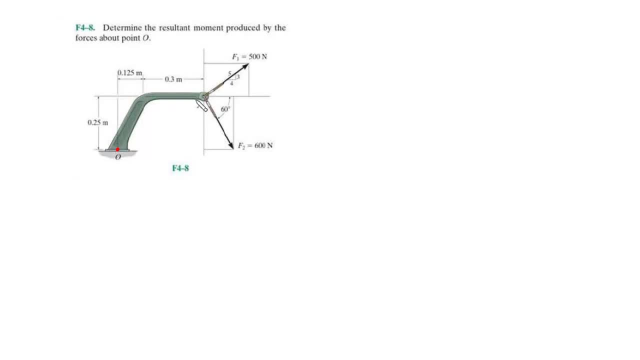 we are given a small slope triangle And then we are going to determine the x and y components of F1. So let this one be the x component, So that is F1x. You have this to be the y component, which is F1y. So for F1x, to find the value of F1x. 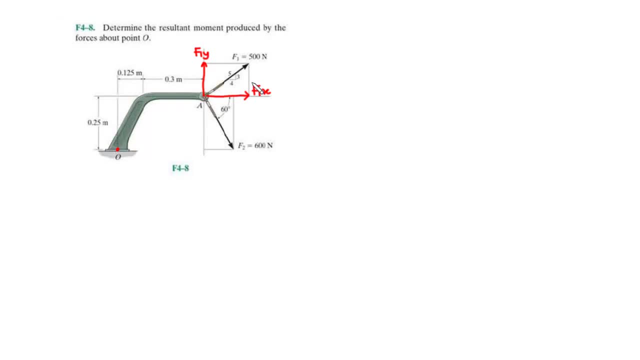 you know that F1x corresponds with 4.. Therefore, you have F1x over 4 equals F1 corresponds with F5. So you have F1, which is 500 divided by 5. And then F2 is the value of X and Y. Then you know that F1x corresponds with 4.. Therefore, you have F1, x over 4. this is the value of X, So for that F1xt corresponds with 4.. Therefore you have: F1x91 is less than or equal to 0.. Damit W- Forget about category Swan's like 5 or X- is either this: 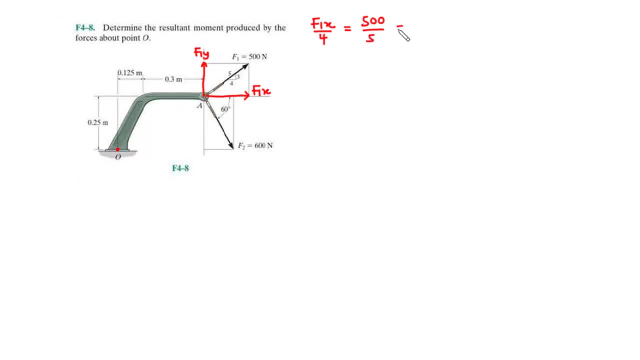 by 5.. Therefore we have: F1x equals 4 times 500 all divided by 5.. 5 goes here once, 5 goes here 100 times. Therefore, 4 times 100 is equal to 400 newtons. So that is the value of F1x. 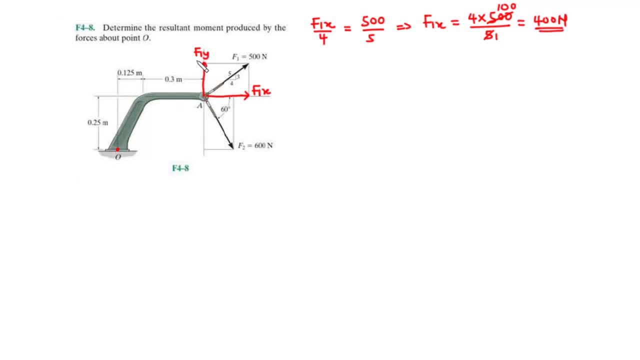 Now also for F1y. you know, F1y corresponds with 3. So we have: F1y divided by 3 equals F1, which is 500 newtons corresponds with 5. So that is 500 divided by 5.. 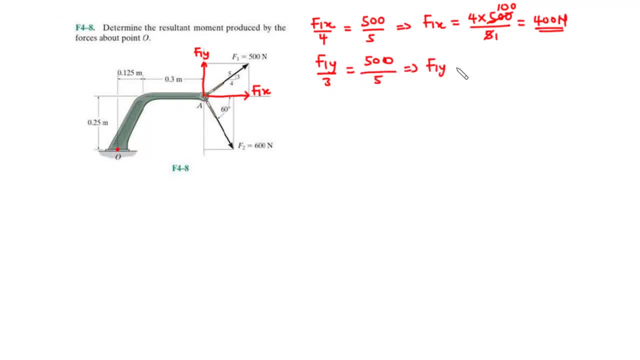 And then we have F1y equals 3 times 500 all divided by 5.. 5 goes here once into 500, 100 times, and then 3 times 100 is 300 newtons. So these are the values of F1x and then F1y. 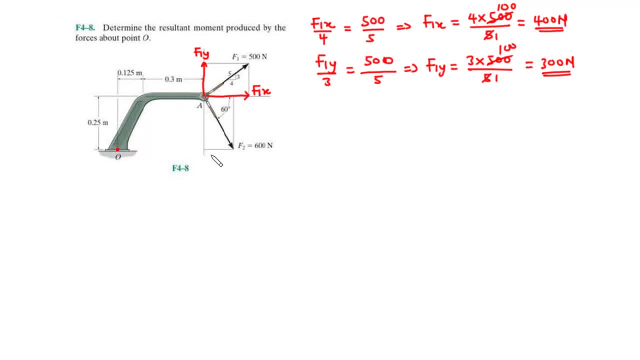 Now let's also resolve F2 into its X and Y components. So we are going to have this to be and then that to be F2Y. So for F2X, that is going to be 600 times cosine of this angle. 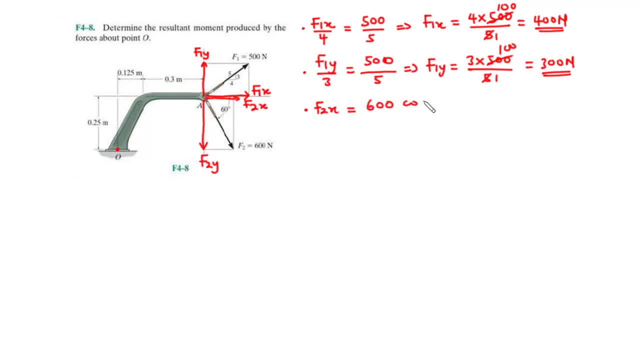 So 600 cos 60, and then F2Y becomes 600 sine 60.. So 600 cos 60 is 300, and then 600 sine 60 is 519.6.. So these are the values of F1X, F2X, F1Y, F2Y. 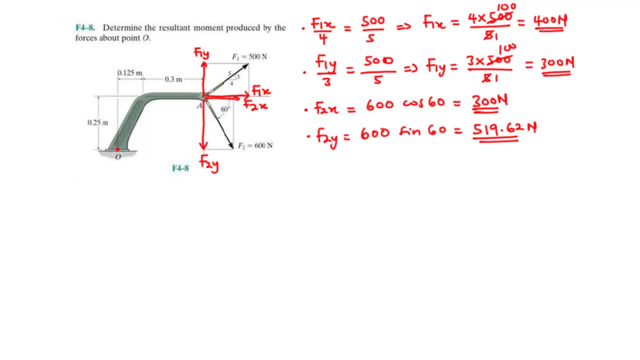 Now let's find or determine the resultant moment produced by these forces about O. So that is MO equals. So for F1X, the perpendicular distance from O to the line of action of F1X is this distance, which is 0.25 meters. 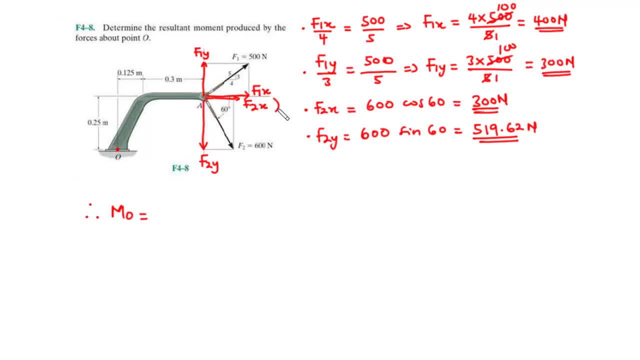 And then we are going to take the moment in the clockwise direction for F1X, So that's going to be positive. So we have F1X, which is 400 times the perpendicular distance, which is 0.25 meters, And then for F1Y, this is F1Y, and then the perpendicular distance from O to the line of action of this force. 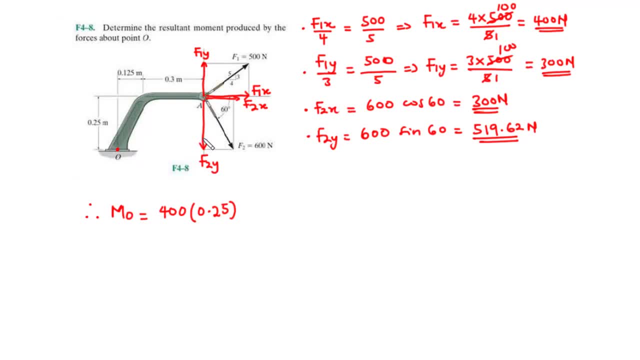 is going to be so. the perpendicular distance is going to be this, And that's going to be 0.125 plus 0.3, which is 0.425.. Now, because we are going to take the moment in the anticlockwise direction, that's going to be negative. 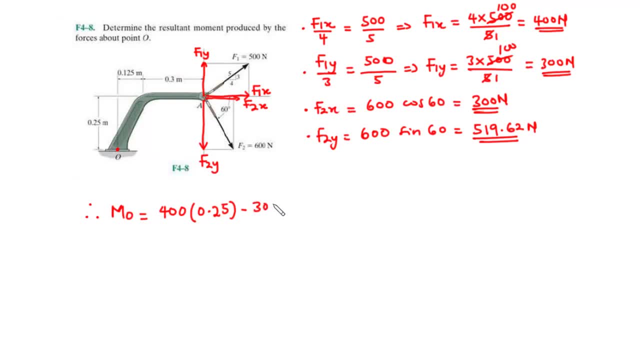 So minus 300 times 0.425.. And then for F2X- this is F2X- the perpendicular distance from O to the line of action of F2X is also 0.25 meters. And then we are also going to take the clock. 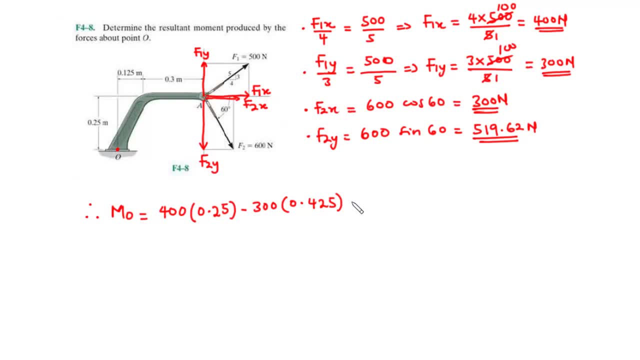 So we are going to take the clockwise direction. So it becomes positive. So positive 300 times 0.25.. And then for F2Y, the perpendicular distance from O to the line of action of F2Y is going to be this distance. 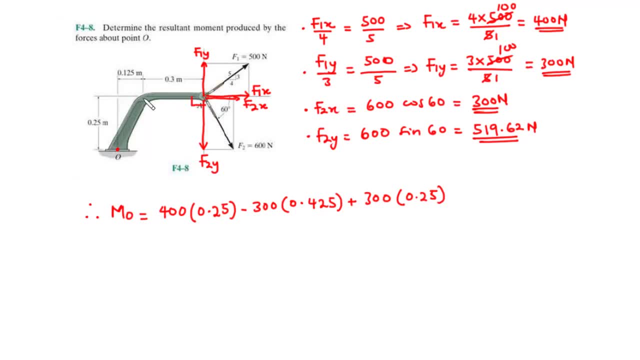 So 0.25.. 0.125 plus 0.3.. So that is 0.425.. And then the moment is going to be taken in the clockwise direction. So positive. So plus 519.62 times 0.425..